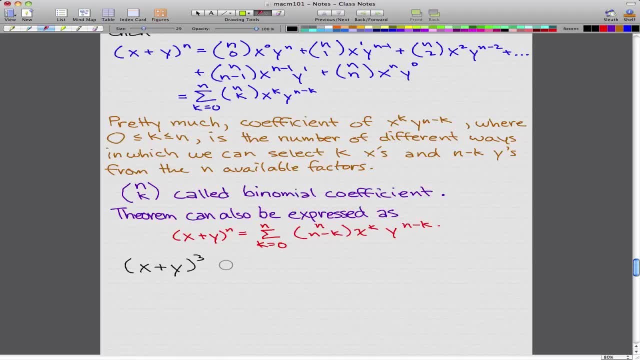 now, if you want to get a certain coefficient of a certain uh x to the power of something and wider power of something, then we'd probably have to expand it out like so x plus y, x plus y, and then we'll take like and then we'll do FOIL and then we'll expand this. 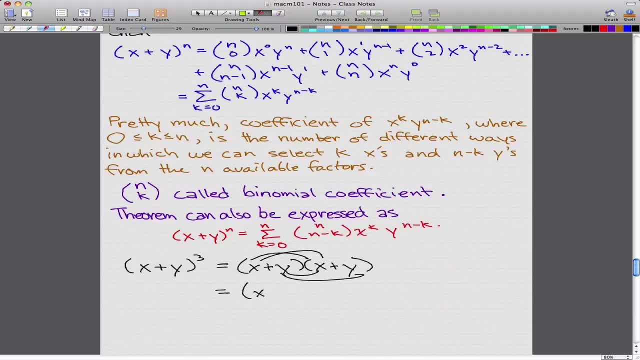 so timesing them all together, we'll get something like x to x to the power of two plus two times x, y plus y squared. but then again we have another x plus y. so then that leaves some more work for us to do. so we'll have to times it by x and y again and expand it, which will 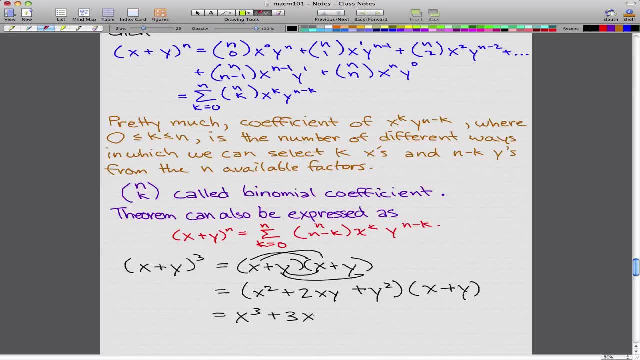 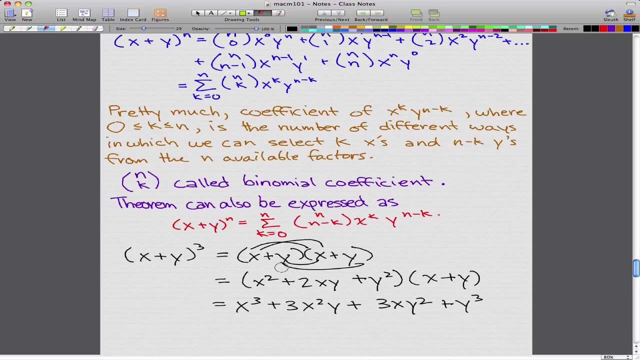 come up with x cubed plus three, x squared y plus three, x y squared plus y three. now, let's imagine that I told you to uh. well, let's imagine that I made the, I made the uh, I made this to the power of a hundred. then you'll have to expand this a hundred times and that is a really a lot of work. 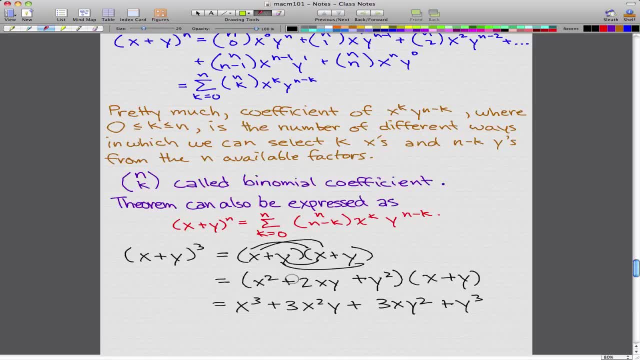 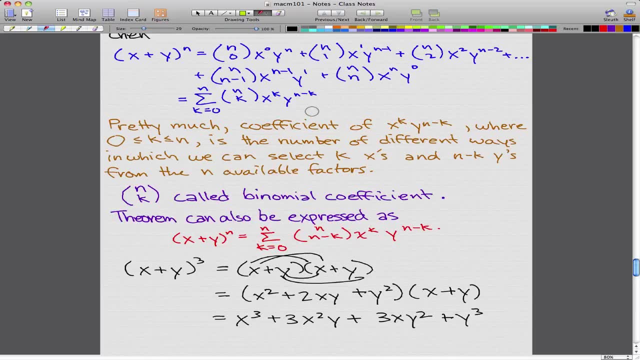 and if I told you that I want the coefficient of, say like x to the power of 97, y to the power of 3, then that's a lot of expanding you have to do. that's where the binomial coefficient comes in. this is where the binomial theorem does its job. 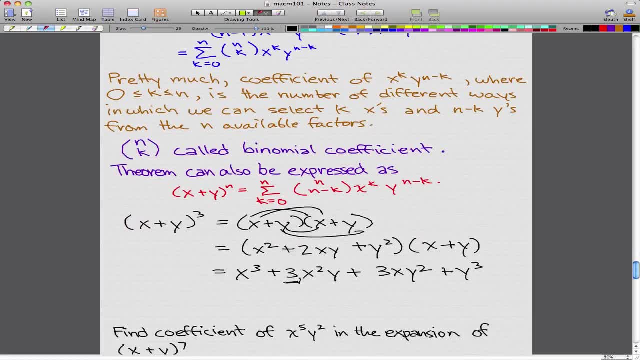 it helps you get the coefficient like the, and this is the coefficient right. this is what we call the binomial coefficient. using that formula, we can get this number anytime without really expanding the entire equation. that really takes a lot of work in which you don't want to do. 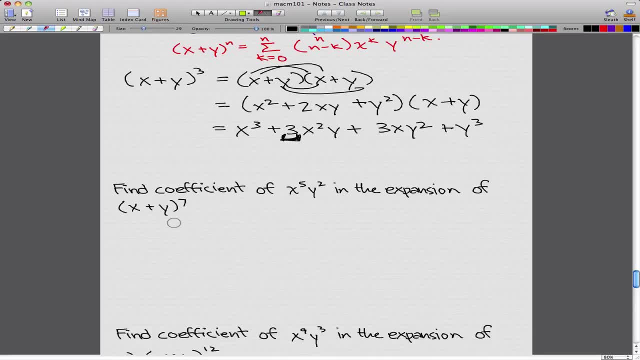 so let's just go through an example of how we actually do this. and let's say: find the coefficient of x to the power of 5, y to the power of 2 in the expansion of x plus y, 7.. so this is really simple. 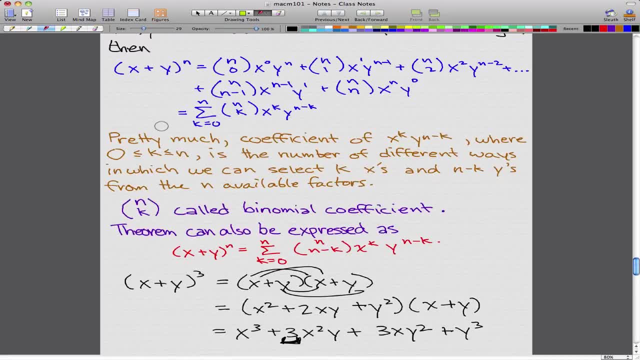 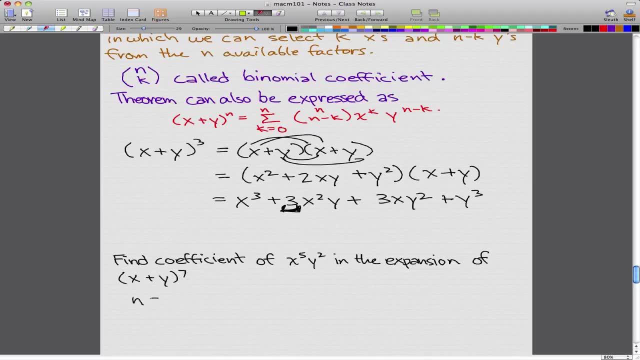 it's pretty much using this formula all over again. so so x plus y to the power of 7. well, 7 is actually our n, 7 is our n is actually our n and our k- we could say our k- is five, because what we're doing is we're following.